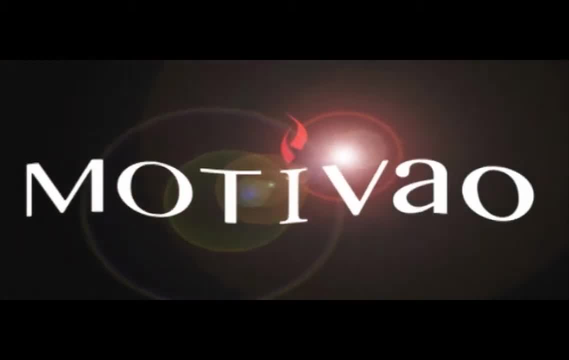 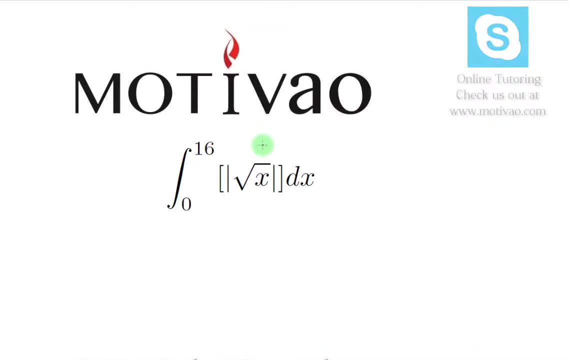 How's it going, guys? This is Joshua from MultiVal Online Instructors, and today I'm going to do the integral from 0 to 16 of the floor function of the square root of x- dx. Now things are going to get a little more interesting. Now, like always, let's go straight to the definition. 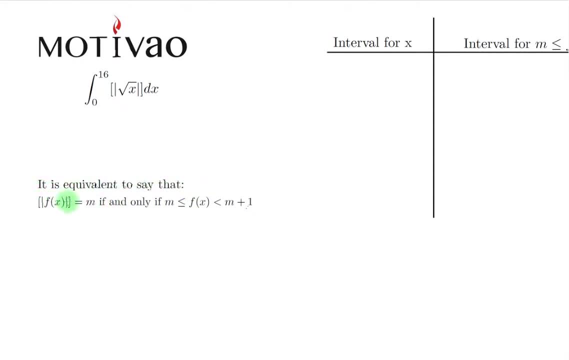 It is equivalent to say that the integer of f of x equals m if, and only if, m is less or equal than f of x, less than m plus 1.. And in this case f of x is equal to the square root of x. And let's do our little table. We already know the square root of x here. 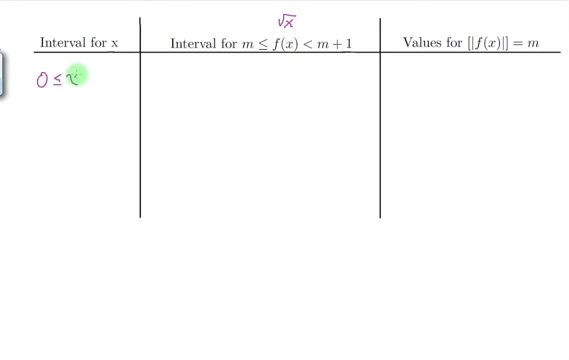 And we start in 0.. Less than 0.. Less than 0.. Less than what? Okay, So remember that the values here affect the values here. What is the square root of 0? 0.. So square root of x, less than, And we always have to add 1.. 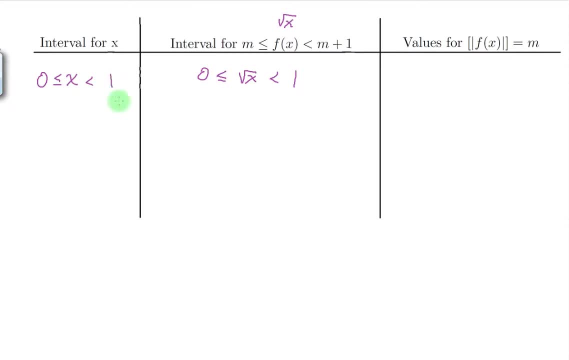 So this is 1.. But what is the square root of 1? 1.. Okay, Now, things are easy now, But let's complicate it a little more. So we go from 1 to square root of x, 2. Because we have to add 1.. But here we start in 1. But we go to where? How do I get? 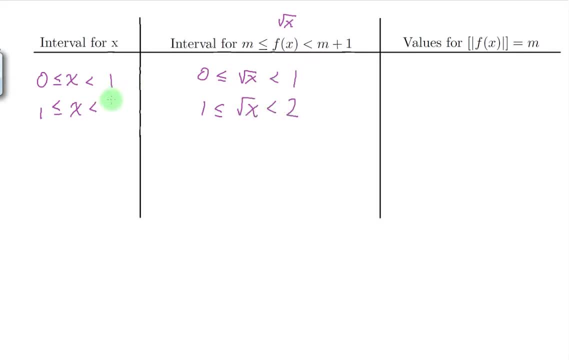 square root of x being 2?? Well, x has to be 4.. Okay, So you see that this jump is in favor of the values here for f of x, So let's keep going. Now we go from 2. And 3.. 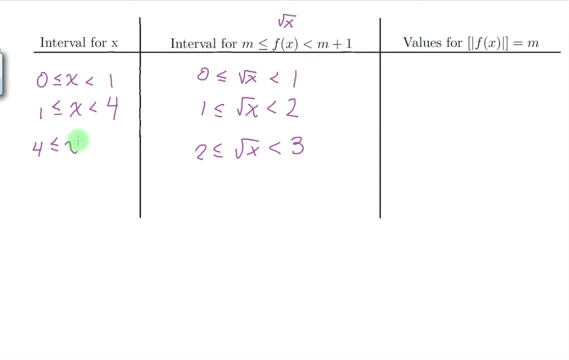 Now we started in 4.. And the question again is: how do I get 3?? Well, we got to go from 4 to 9.. Okay, And we keep going, because the last term is in the x. So this is 3. And 4.. 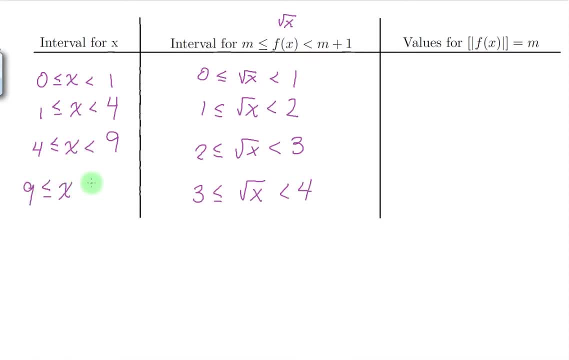 And here we started in 9.. Less than what. Well, to have. 4,. the value is in 4.. And here The value in x has to be 16.. And that's the last value, And here the values are 0,, 1,, 2,, 3.. 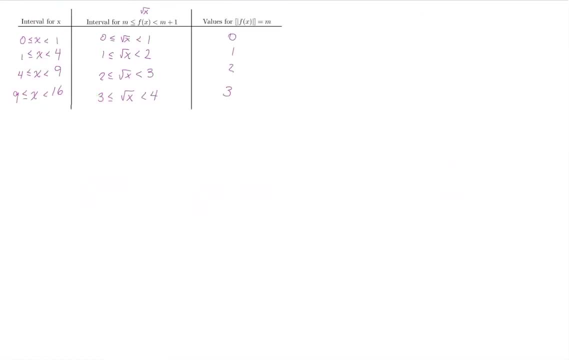 So our integral will look like this. It's going to be the integral, from 0 to 1, of the square root of x Plus from 1 to 4,, square root of x from 4 to 9, and from 9 to 16.. 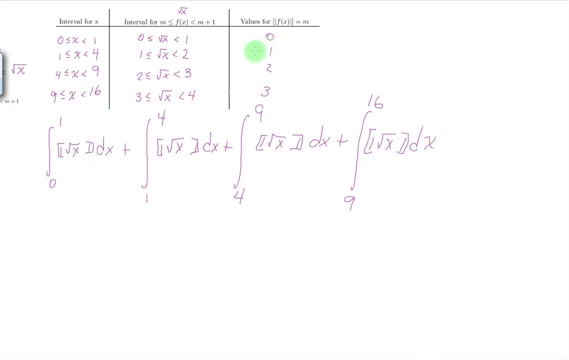 Okay, And now in this interval, the value is 0.. So we have from 0 to 1, we have 0.. From 1 to 4, we have 1.. From 4 to 9, we have 2.. 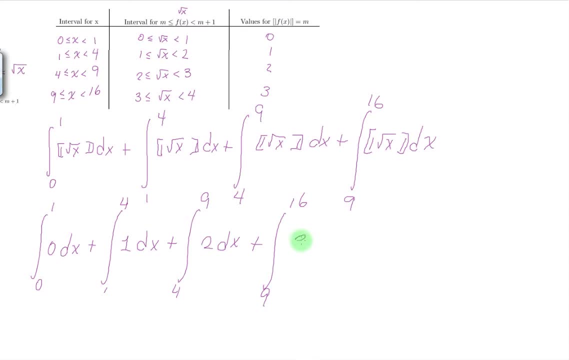 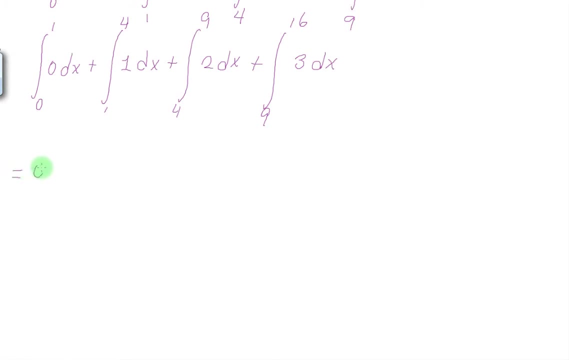 And from 9 to 16, we have 3.. Okay, Now we evaluate the integral. This becomes: 0 times x evaluated from 0 to 1, plus 1 times x evaluated from 1 to 4, plus 2x evaluated from 4 to 9, plus 3x evaluated from 9 to 16.. 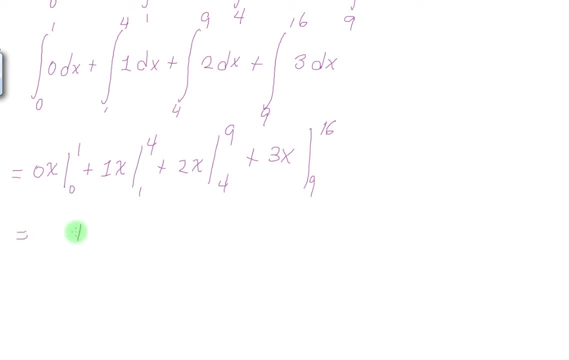 And this is equal to 0, plus 4 minus 1, plus 2 times 9, minus 4, plus 3 times 16, minus 9.. This is equal to 3, plus 2 times 5, plus 3 times 16, minus 9 is 7.. 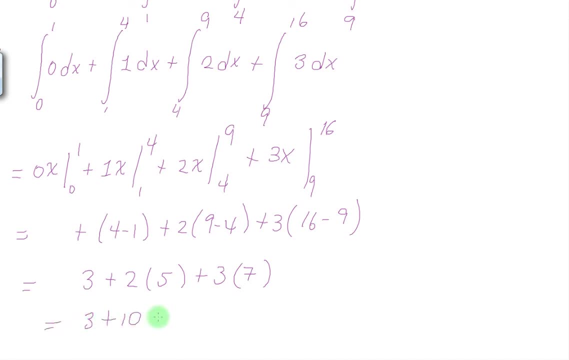 So this is equal to 3 plus 10, plus 21,, which is 31.. 31 plus 3 is 34.. And that's our answer, guys. Thanks again for watching. and this is Joshua from Motivau.